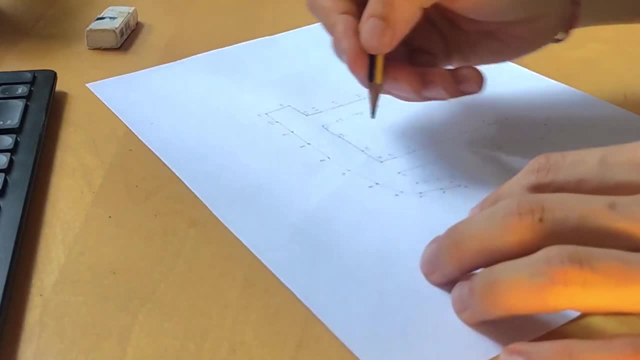 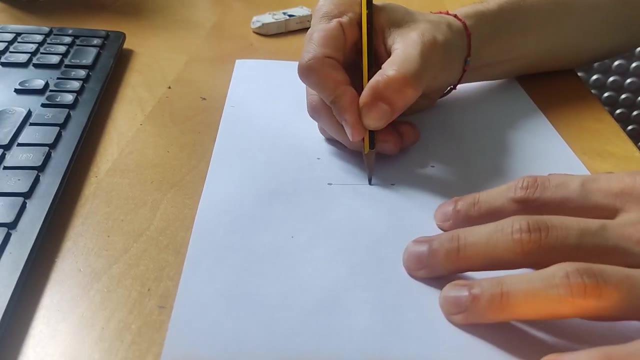 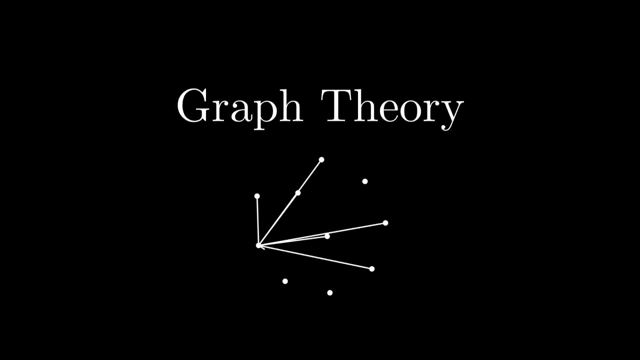 When I was a kid I used to love those connect the dots thingies, and the thing I would do in my spare time during art classes was draw a bunch of points and try to connect each dot with every other dot. Well, I would discover much later that that game I used to play was the very first instance of graph theory in my life. 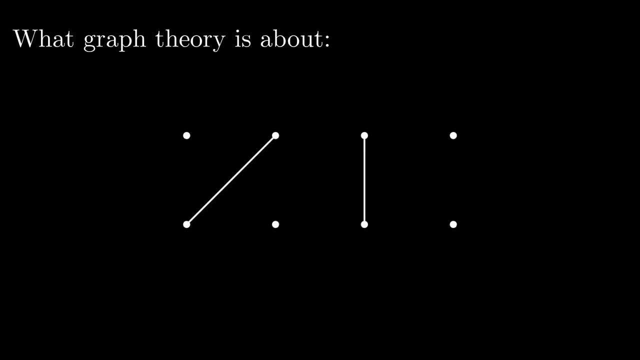 Graph theory has nothing to do with these nasty things. It is the art of dots and lines that make pretty patterns, And its simple basic elements, that is, dots and lines, are enough to find lots and lots of different applications. A graph is a pair, VE, where V is a set of vertices and E is a set of edges, represented as pairs of vertices. 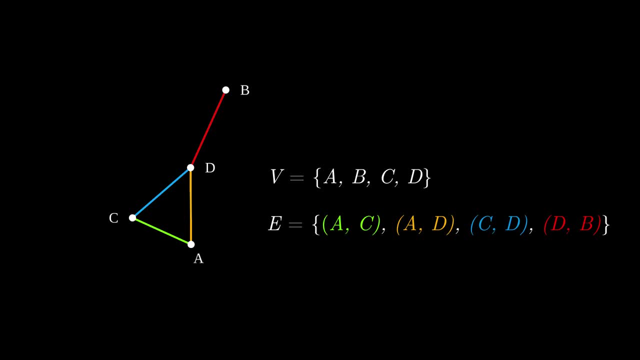 Vertices and edges is just a fancy way of saying dots and lines. I hope this definition makes sense. In particular, I hope you're comfortable with the representation of edges as pairs of vertices. I'll give you a few seconds to think about that. 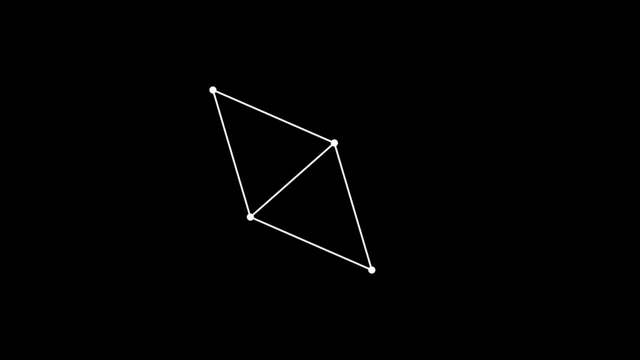 The game I used to play as a kid is called Construction of the Complete Graph, And complete graph is just a name of a graph that has an edge from every vertex to every other vertex. A graph with no edges from any vertex to any other vertex may well exist, and it is called an empty graph of order n, where n is the number of vertices it has. 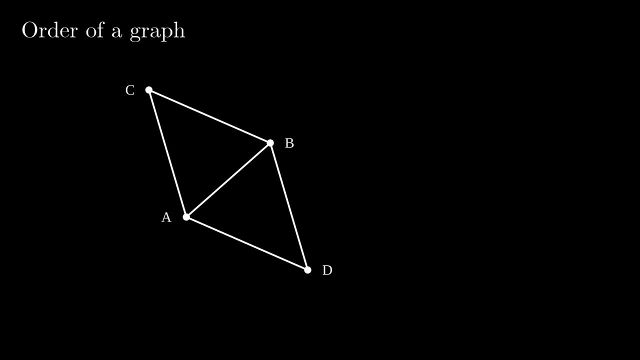 In general, when we refer to the order of a graph, we are talking about its number of vertices. A graph may also be directed, That is, we may draw an error from A to B and say that A is connected to B but B is not connected to A, unless there is another error from B to A. 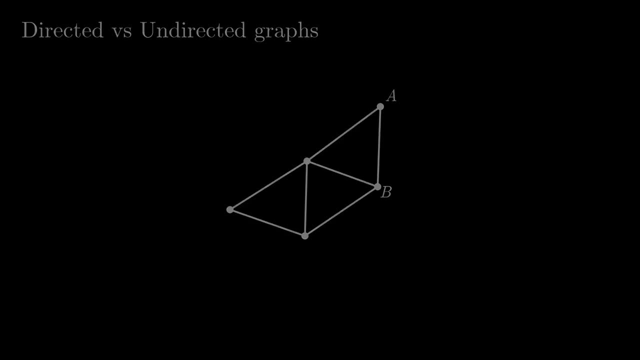 We'll just focus on undirected graphs for now. The next thing I'd like you to think about is: what does it mean for something to be the same as something else? Are these two the same? Well, yeah, they're both triangles, but they're not the same triangle. 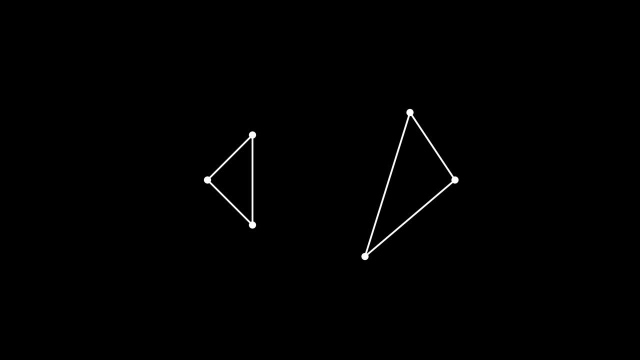 The lengths and angles are all different, so they're not the same. But what happens if we assign names to the vertices of these triangles in such a way that their graph representation is the same? Are these the same triangles? No, Are they the same graph? 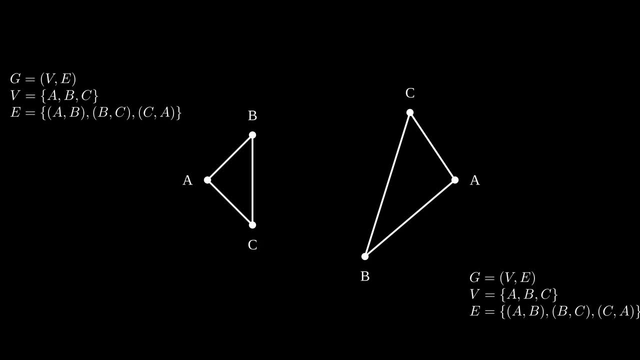 Yes, So in order to be the same, two graphs need not be the same shape. they just need to have the same number of vertices and the same edges. That is, for all couples of vertices A and B, they need to have the same number of vertices and the same edges. 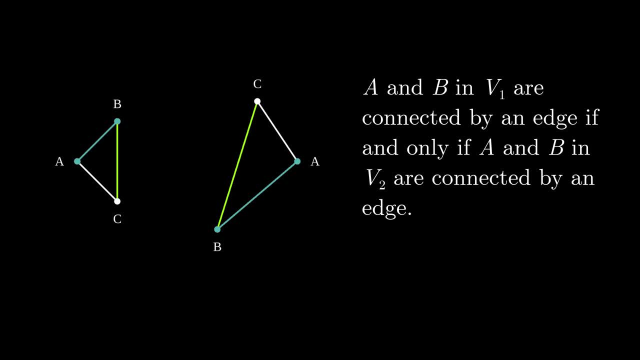 For all couples of vertices A and B. the vertices A and B in one graph are connected by an edge if, and only if, the vertices A and B in the other graph are connected. And this could be a satisfactory definition, but it ignores a simple idea. 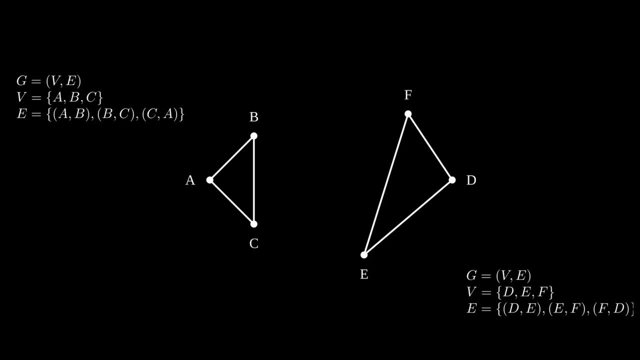 What if we were to call the edges of the triangle on the right with different names? Are they the same graph now? Well, the previous definition does not make any sense right now, But I think they should be the same graph. they deserve to be the same graph and that's because they have the same structure. 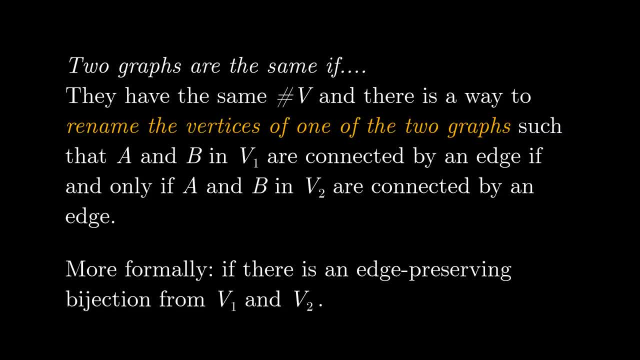 So let's rewrite the definition. Two graphs are the same if they have the same number of vertices and the same edges. That is, there exists a way of renaming the vertices such that for every couple of vertices- A and B- the vertices A and B in one graph are connected by an edge if, and only if, the vertices A and B in the other graph are connected. 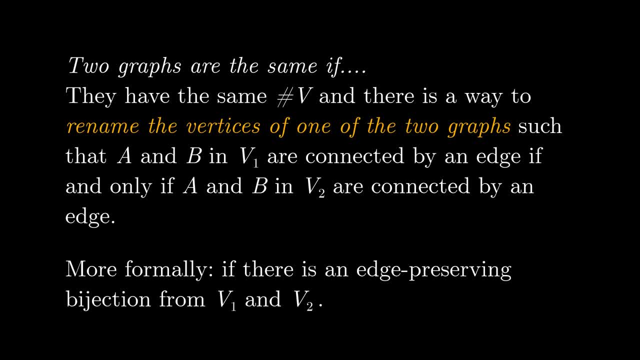 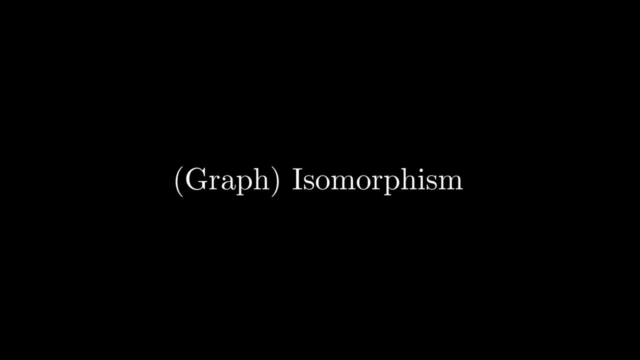 And that is when two graphs are the same. We don't care about names and shapes, just structure. This special kind of sameness is called isomorphism, and it's a very important concept in mathematics. I will now show you a few graphs and let you try to figure out whether they're isomorphic or not. 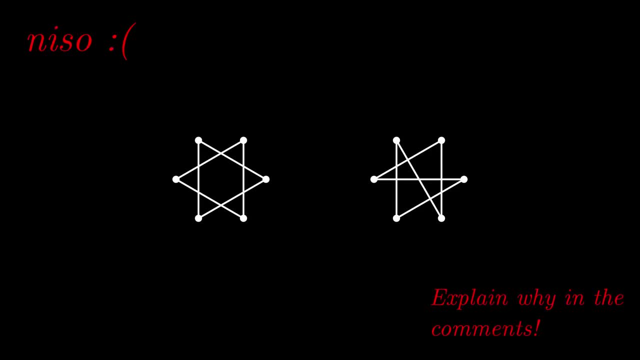 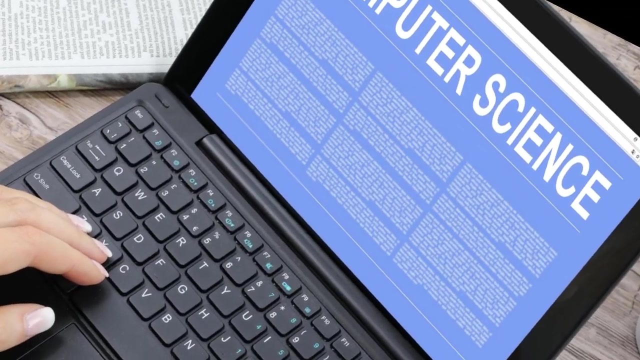 An actual lesson on graph theory would now start describing planar graphs, Euler's formula and platonic graphs, And those are interesting and you should Google those terms to learn about those concepts. But I view things from a computer science point of view, so I really, really want to give you an idea of why I find graph theory so powerful. 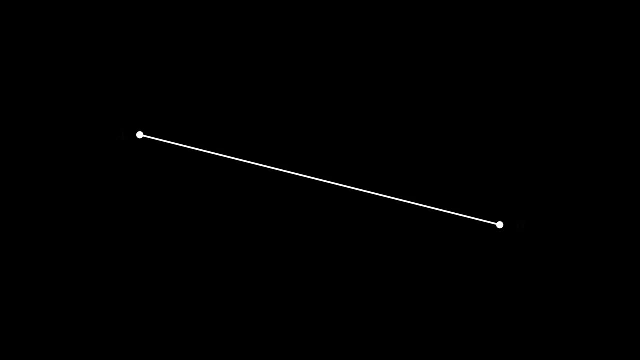 By deciding whether or not A and B are connected by an edge, we are assigning them some sort of a distance. If they are connected, they have a distance of 1. If they're not- but A is connected to a vertex C that is in turn connected to B, they have a distance of 2.. 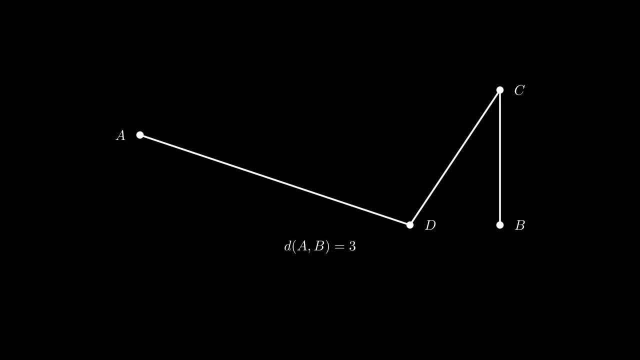 If they're not connected and they don't have a distance of 2,, they might have a distance of 3.. You may think of this as Facebook friendship: A can be friends with B, or they can be friends with some other friends, and so on. 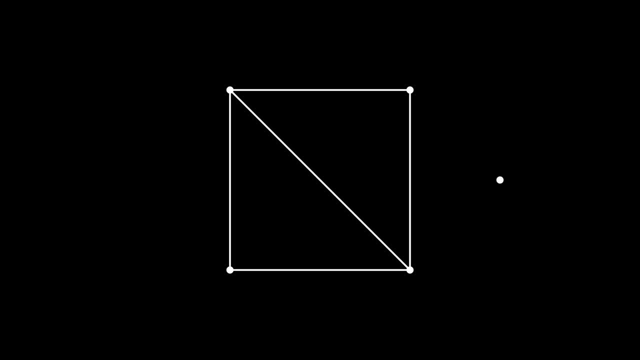 What if there is a vertex that is connected to B. It is not connected with any other vertex? In that case, we may say that that vertex is infinitely far away from the others. This concept of distance is very important for managing big networks, which are graphs, if you think about it. 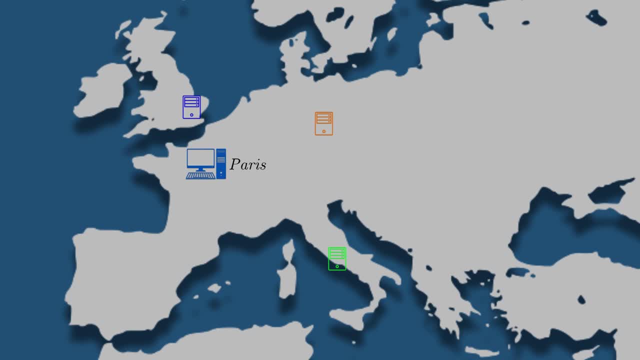 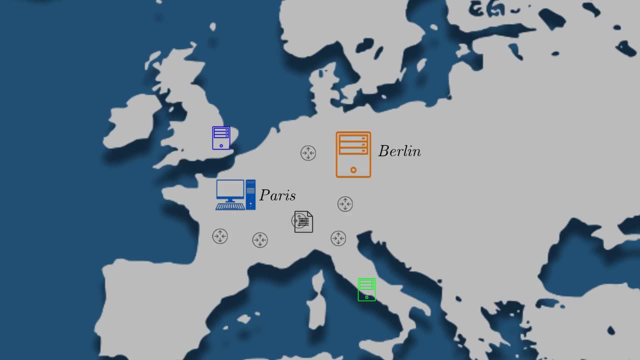 Let's say you're in Paris and you want to download a file. You may not want to download it from a server in Tokyo, You may prefer a server in Berlin, And knowing how many times the signal has to bounce before getting to your computer is crucial for performance. 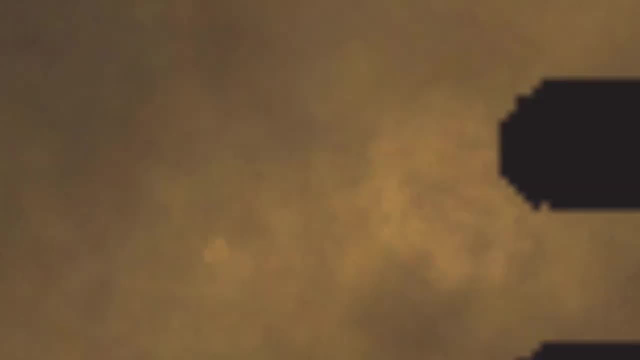 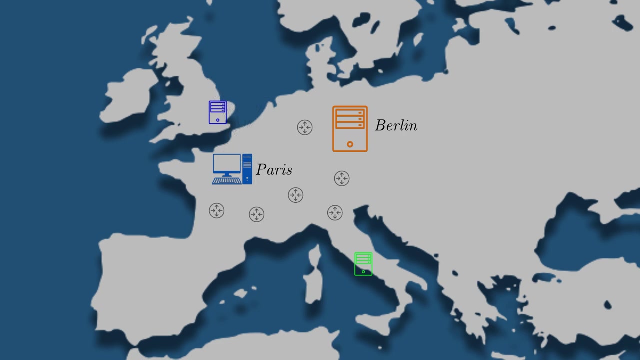 We don't want the file to travel for longer than that. It's unnecessary. Even if you were to pick the closest server, there may be several ways to reach you and some of them may be longer than others. We need systematic ways to find which way is shortest, the so-called shortest path algorithms. 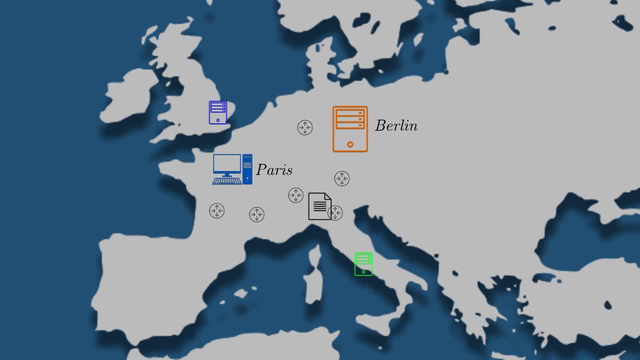 And, although the idea may sound silly, the file may even get stuck if we're not careful enough, because a graph may contain cycles and if we start spinning around in a cycle, we may never get to our destination. Another very important instance of a graph is a tree. 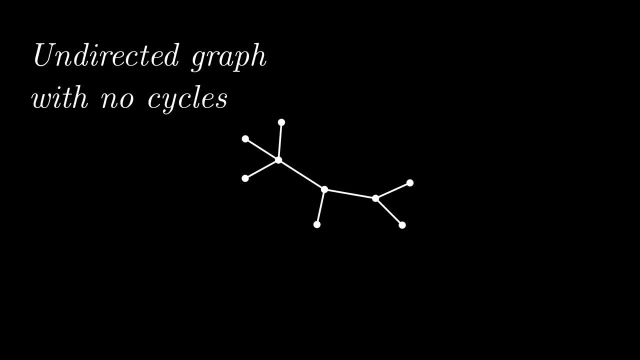 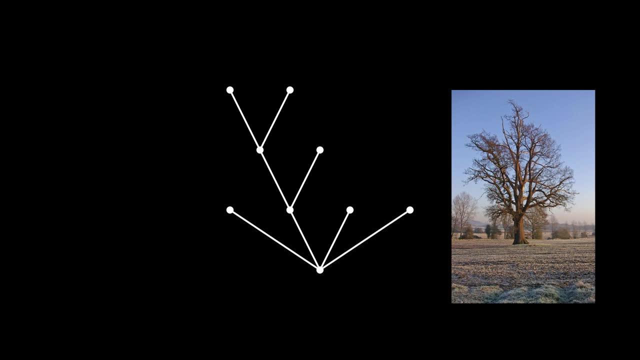 A tree is a graph with no cycles. More precisely, it is an undirected graph with no cycles. It's called a tree because, well, it looks like one. The only thing weird about it is that computer scientists tend to represent trees upside down. 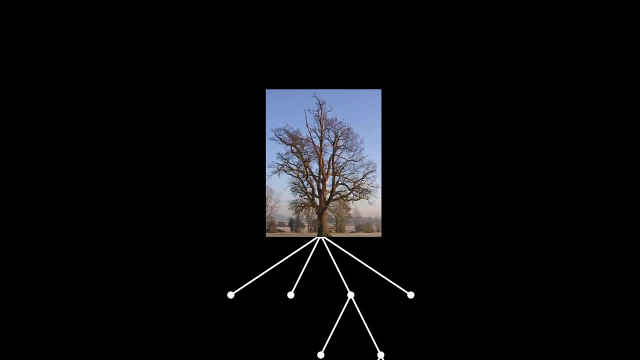 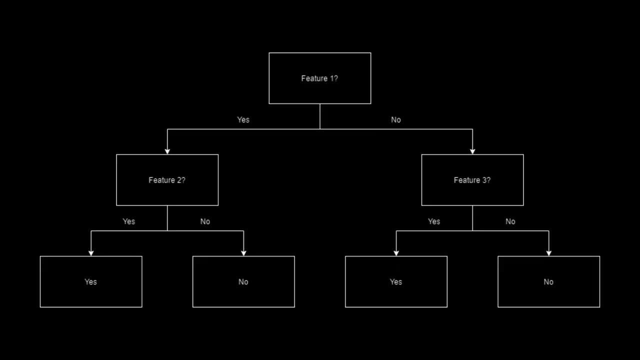 so they look a bit more like roots, but the mathematicians would be very angry if we called them roots. so we had to make a decision: Who to irritate the mathematicians or the biologists? When making decisions, it's useful to draw a tree with all of our possibilities. 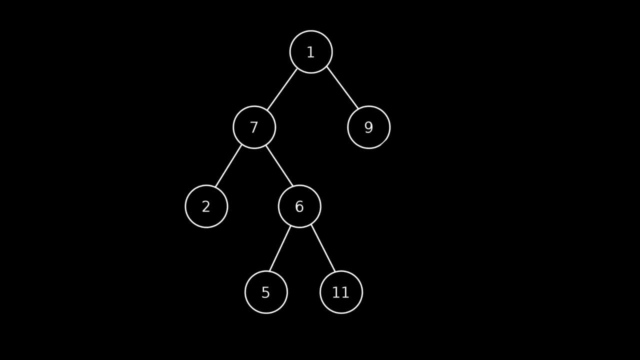 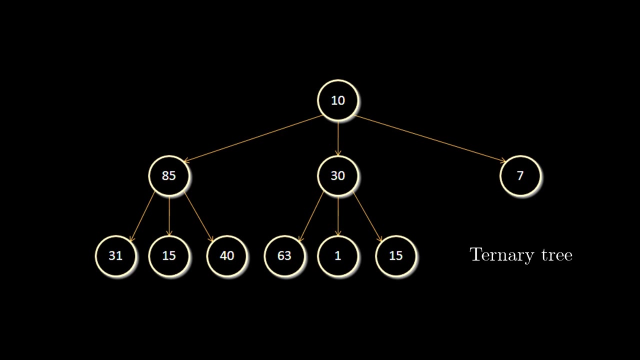 They depend on the choices we make. These may be binary choices, ternary choices, mixed choices and so on. For each of these, we've drawn a tree. A tree that models binary choices is called a binary tree. One that models ternary choices is called a ternary tree. 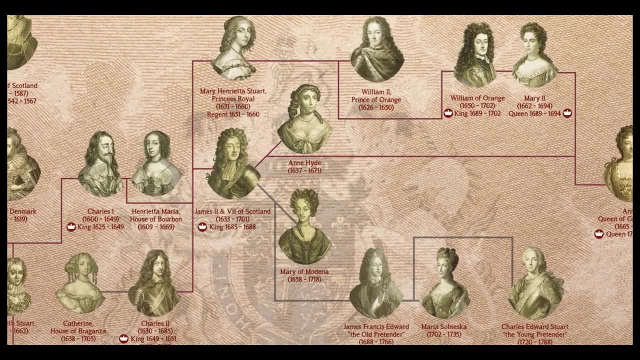 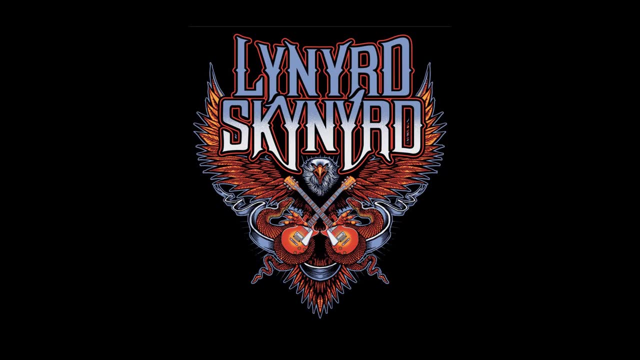 Trees have a lot of other applications. You may know family trees that connect each parent to their children- although they may well not be trees, since there may well be cycles if you live in Alabama- But they're also used as very important parts of compilers and interpreters. 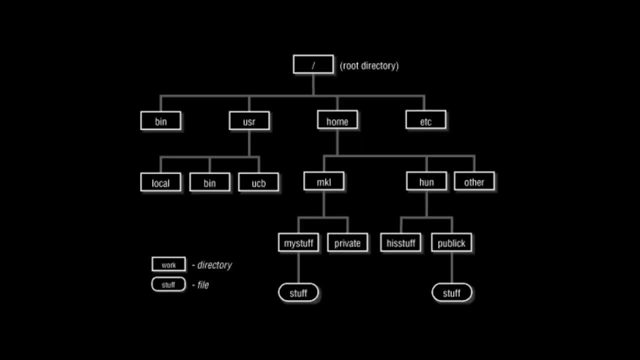 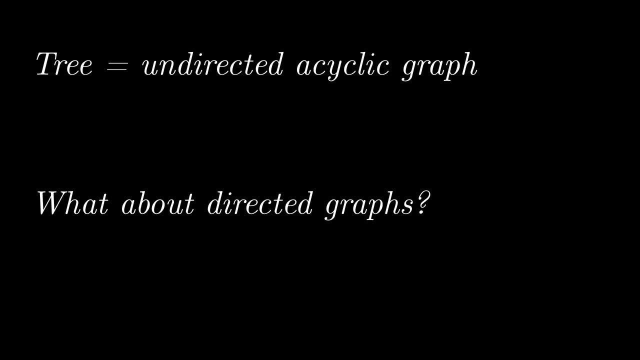 and represent directories and files in a file system. I mentioned that a tree is an undirected graph with no cycles. What would a directed graph with no cycles look like? Well, like this, If you imagine this as some sort of canal system. 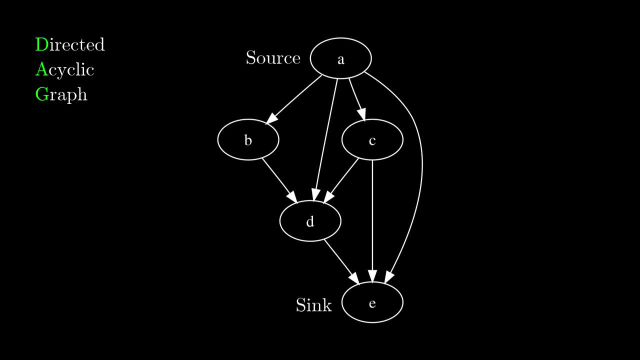 some vertices only have outgoing flow and some others only have ingoing flow. As you might imagine, this is very useful in some branches of economics and optimization theory, But that's a whole other story and I won't go into the details here. 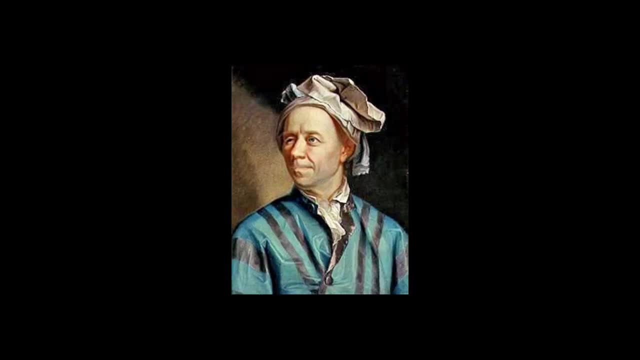 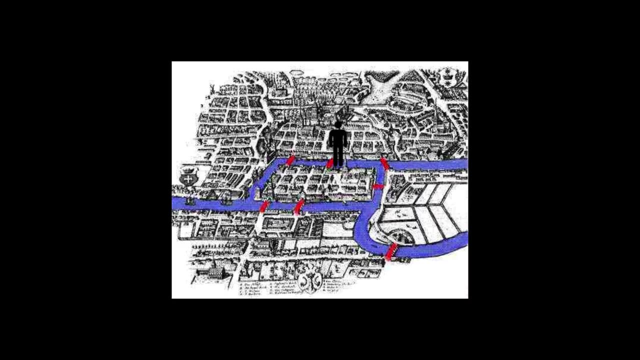 In 1736, a guy called Euler stumbled upon an interesting challenge In the city of Konigsberg. there were seven bridges on a river, And people would try to come up with a path that crosses each of the seven bridges exactly once. 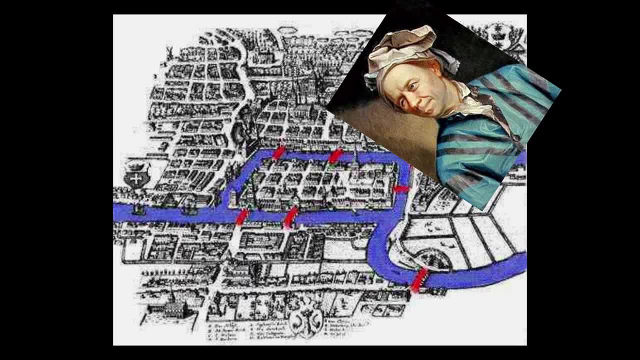 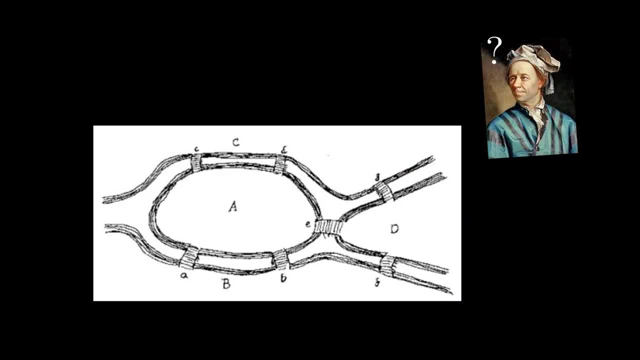 They would try and try, but with no luck. So instead of actually going out there and trying to find a way by walking, lazy Euler drew a map and started to think about a way of abstracting away the bridges, the river and the city. 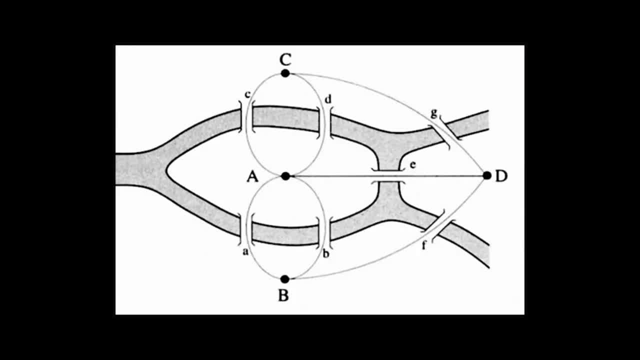 remaining with these regions, which he called A, B, C and D, and the possible ways to go from each region to every other region. So basically a graph. He proved that there is no solution to the problem as it is, but there would be at least one if the degree of each vertex 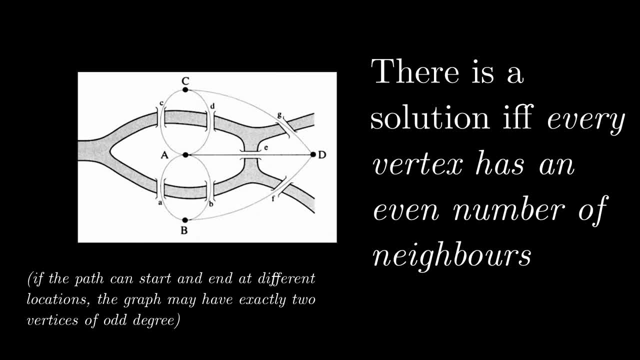 that is, the number of edges that connect that vertex to another, was even. I won't give you the details of the proof, since this is just a brief overview of the subject, but I suggest you to think about why that might be the case. 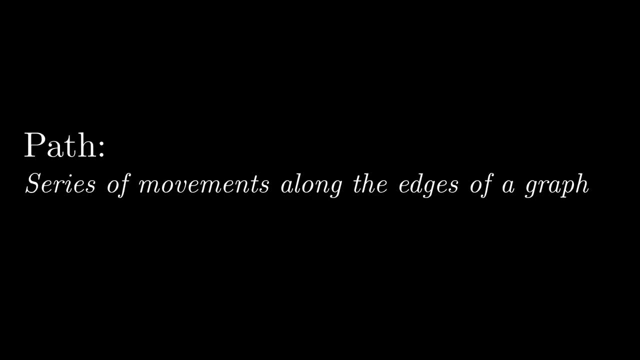 A path on a graph that is informally a series of movements along edges is called an Eulerian path if it crosses every edge exactly once, and it takes its name from the famous problem we just described. A much more complex version of that problem is the following: